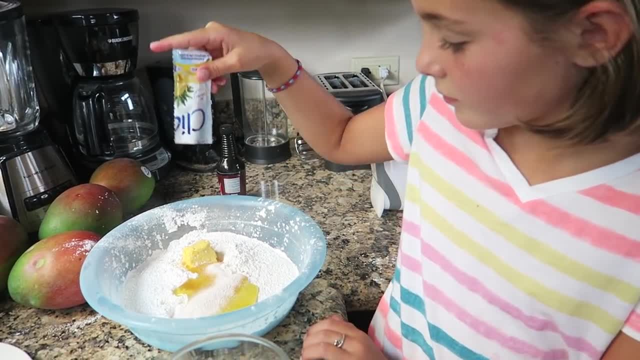 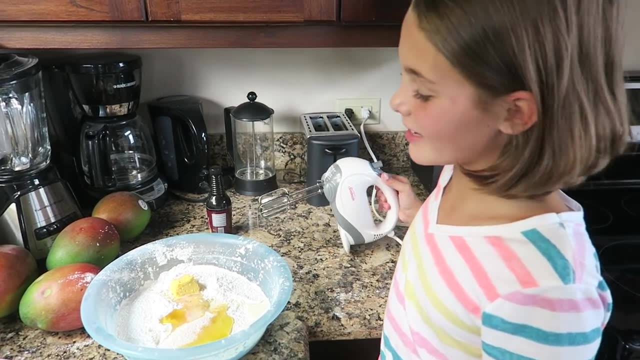 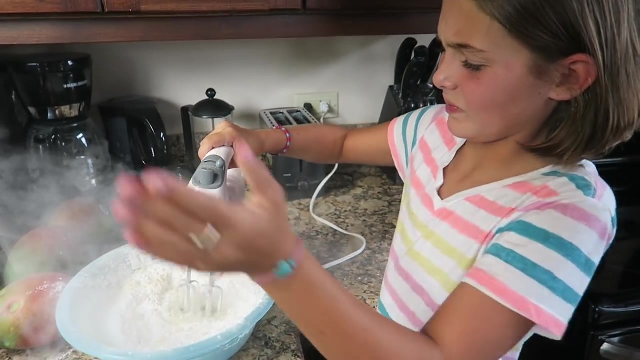 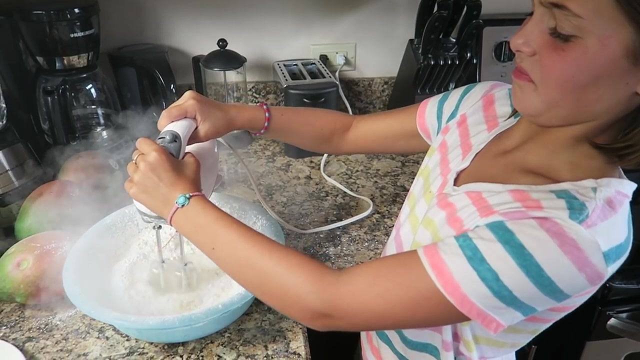 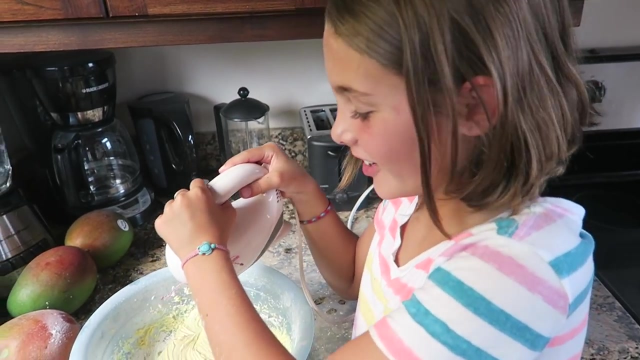 Oh, that smells good. Now I'm just going to add a little bit more sugar. I'm just going to add a tiny bit of milk. All right, let's mix this up. It's like a fog of powdered sugar. Oh yeah, now it's starting to look good. 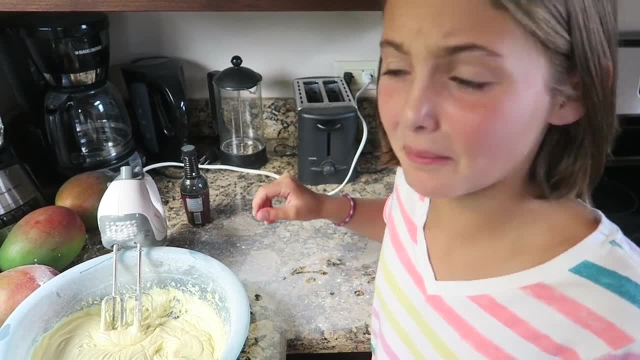 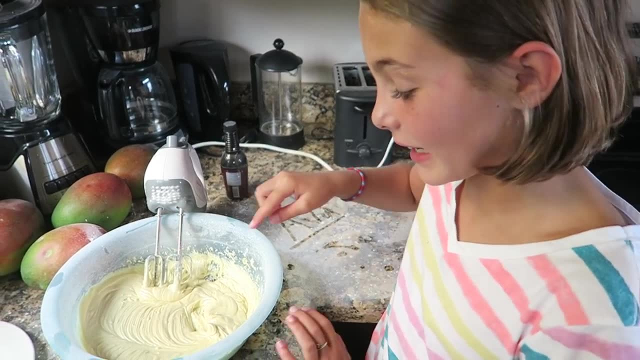 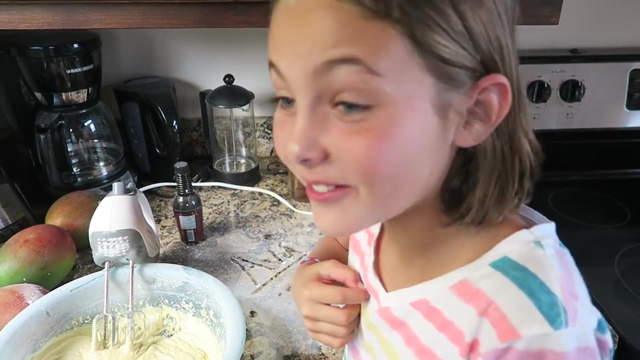 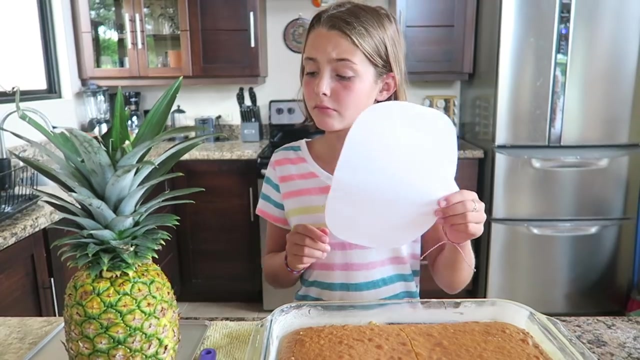 All right, there we go. Oh man, I made a mess. All right, let's taste the frosting and see if it tastes like pineapple. It does, Whoa. Now let's cut out our cake like a pineapple shape. I cut this piece of paper out and it's about the same size as the pineapple. 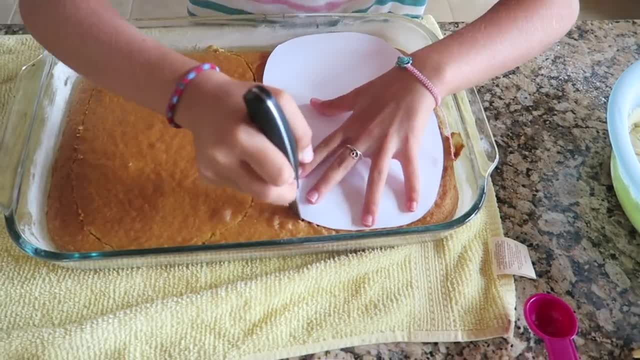 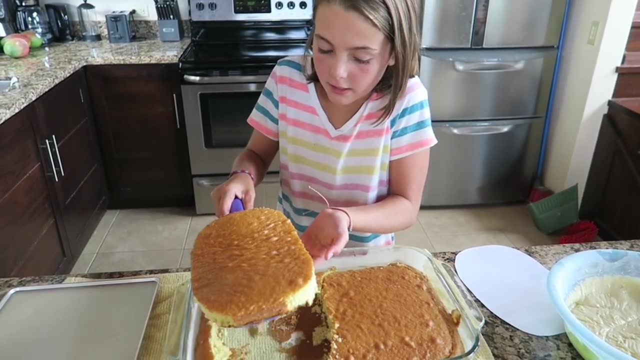 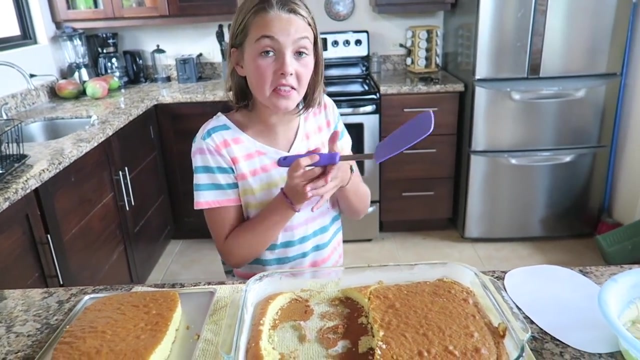 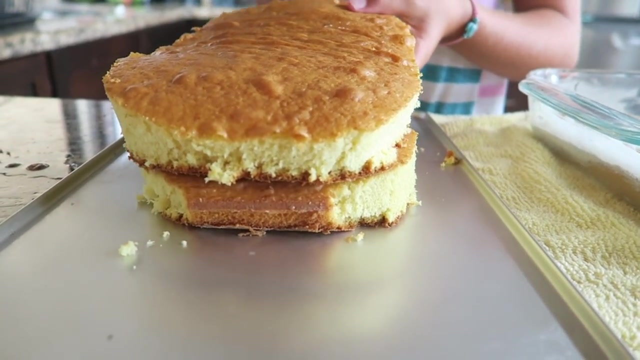 We're going to lay it down here and cut it out. All right, now I'm going to carefully put the cake down There we go. All right time for the next one. Now I'm going to put this right on top of this one. 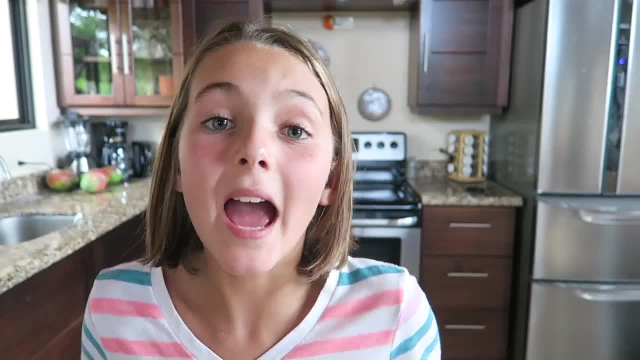 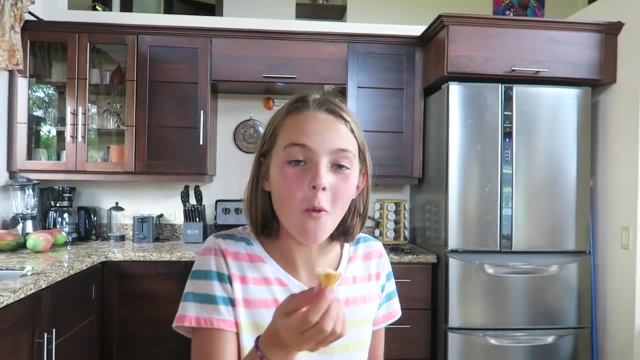 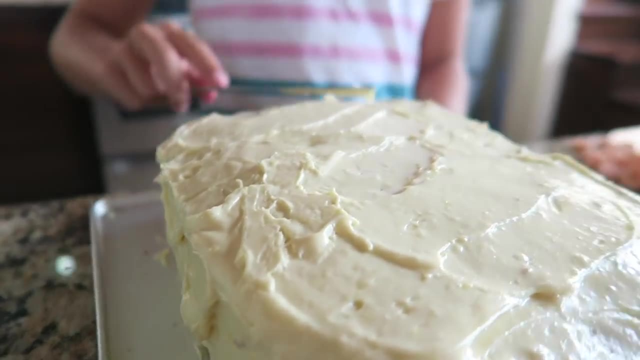 Double decker. And now I get to eat all the scraps for myself. Do you want some? It's good. right Now I'm going to finish frosting our cake with this yummy and delicious pineapple frosting. I've been sorting out these rainbow fruity cereals here. 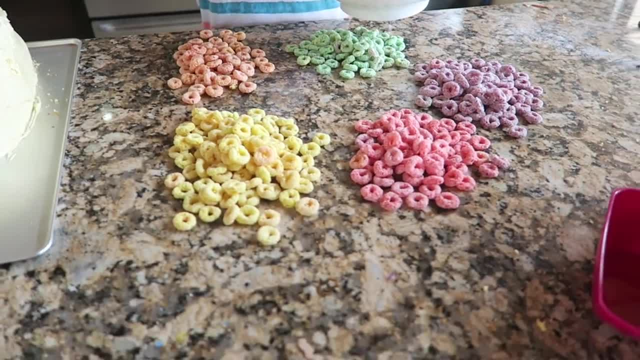 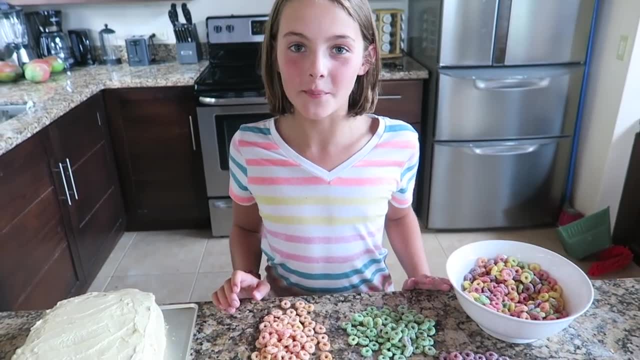 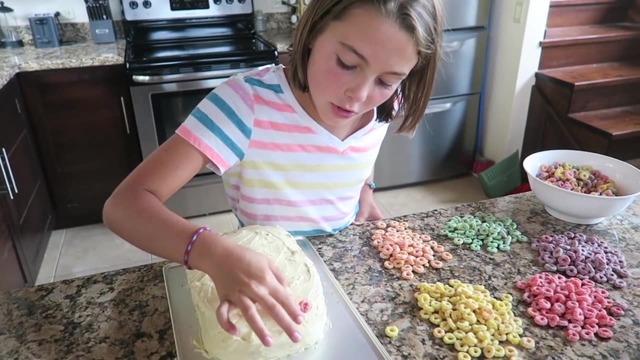 And then we're going to put it on top of our cake: Red, yellow, orange, green, purple. Now comes the fun part. I get to line all of these colors up onto our cake. So I'm going to start with red and just go on to the top, just like this. 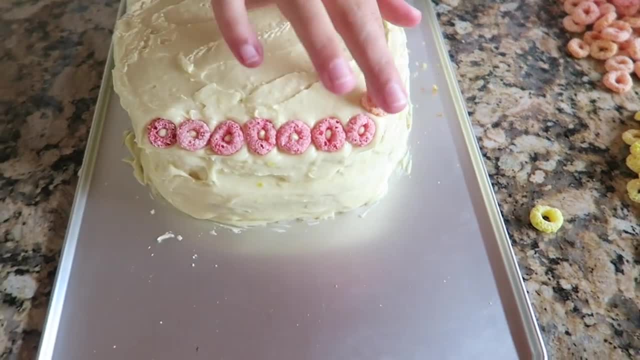 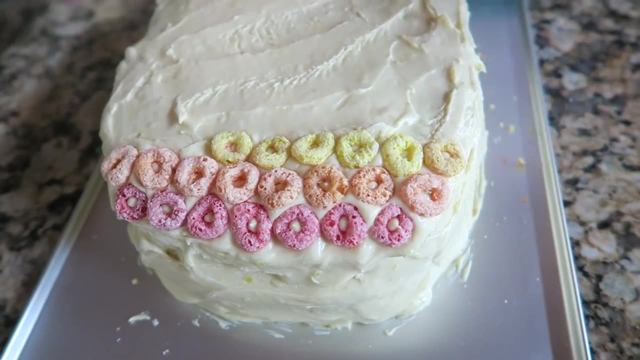 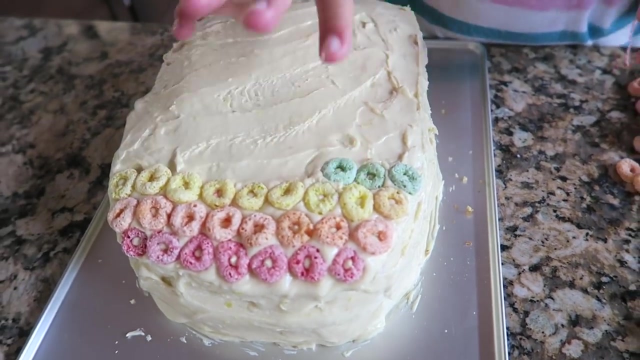 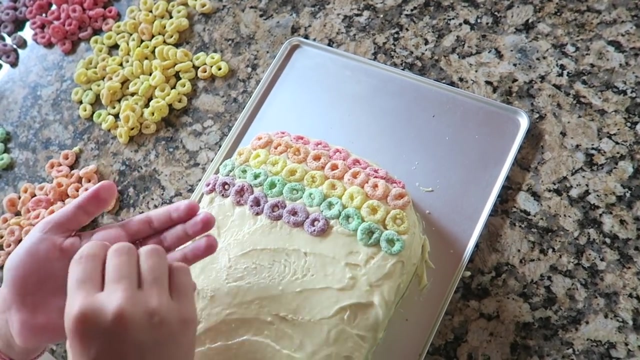 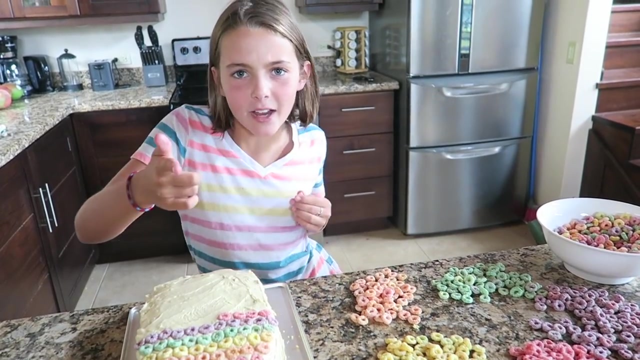 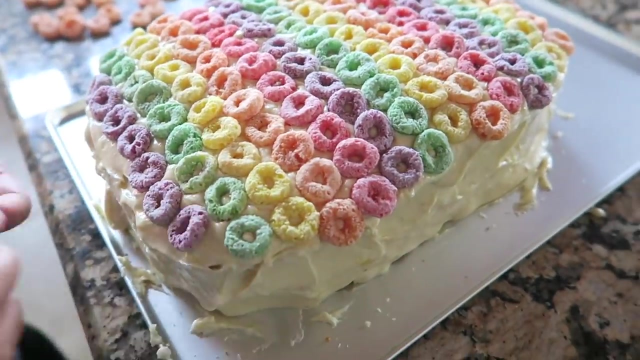 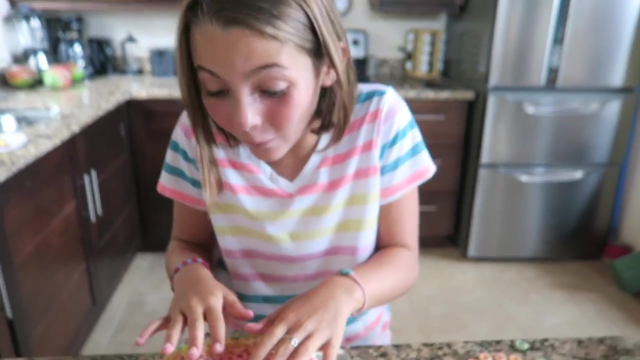 Time for the next color, orange, Next color yellow, Next color green, Last but not least, purple. Now we're going to repeat those colors in order all the way to the bottom. Fast forward now, Ta-da. Oh, this feels so cool. 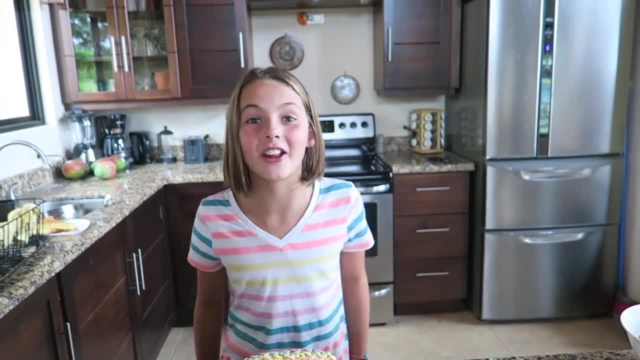 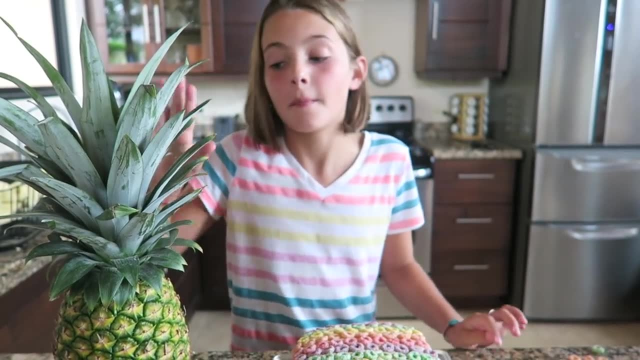 Whoa, Oh, this is going to turn out so good. Now comes the fun part. We're going to take the head of the pineapple off and stick it on the cake. How you do it is just: you grab onto it and you twist. 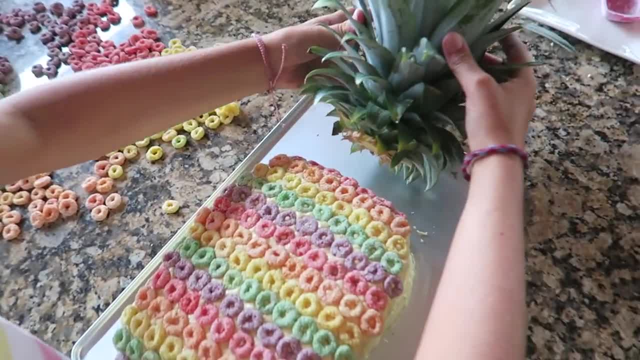 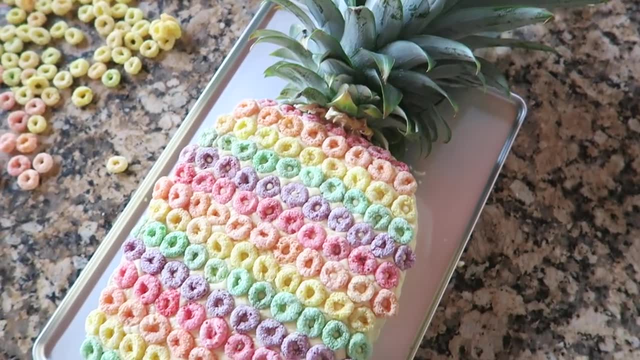 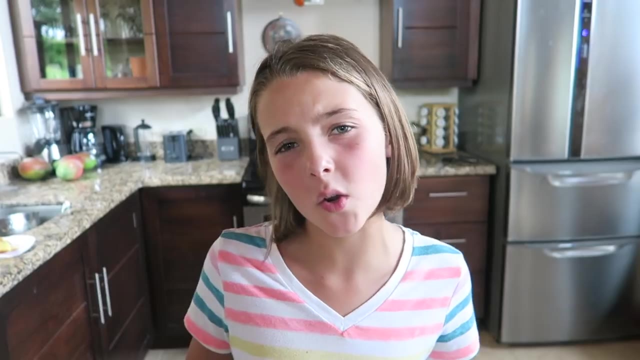 See, And now you put the top of the pineapple onto the cake. Ta-da, Oh, that looks so pretty. Oh, this looks so rad. Whoa, It's a real rainbow pineapple cake. We want our pineapple to be super cool and chill. 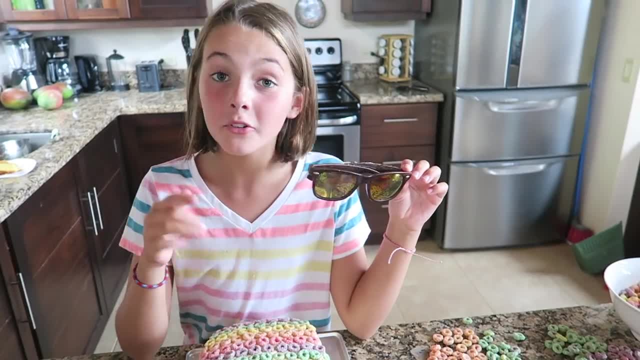 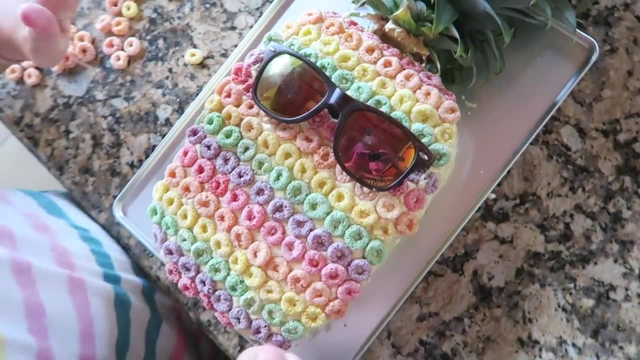 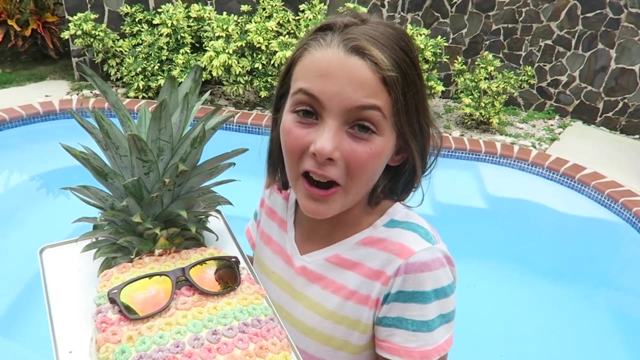 So we're going to put some sunglasses on them. I'm going to remove some of this rainbow cereal and then push these sunglasses into the cake. Oh yeah, there we go. All right, there you have it. Our rainbow pineapple cake is finished. 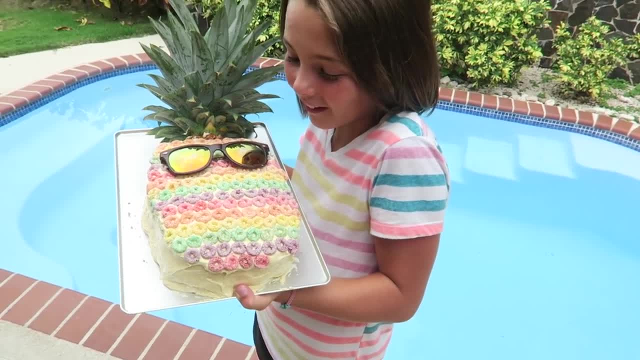 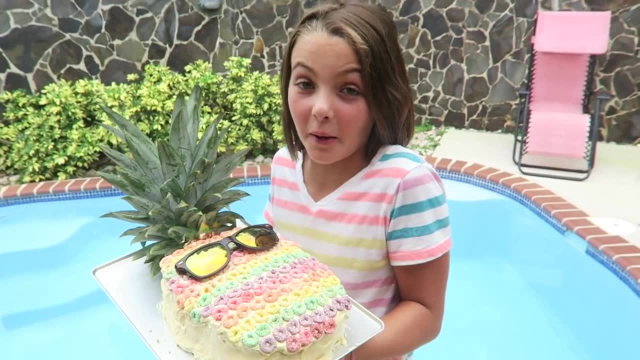 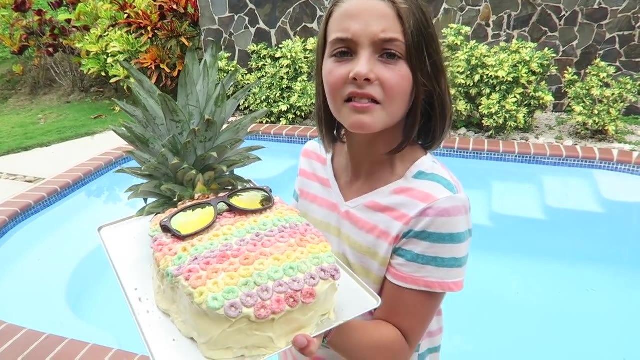 It looks so cool, Guys. I totally realized that this pineapple matches my shirt. I would love this for my birthday Or just for a snack. I could pretty much eat this for breakfast. I mean, it has cereal on it, All right, guys. 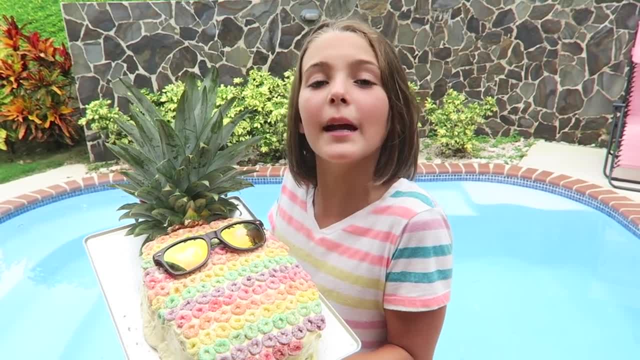 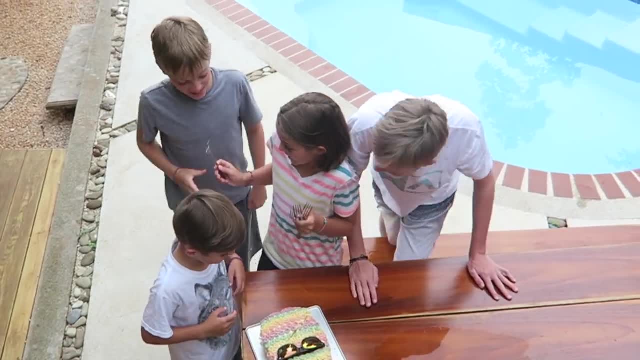 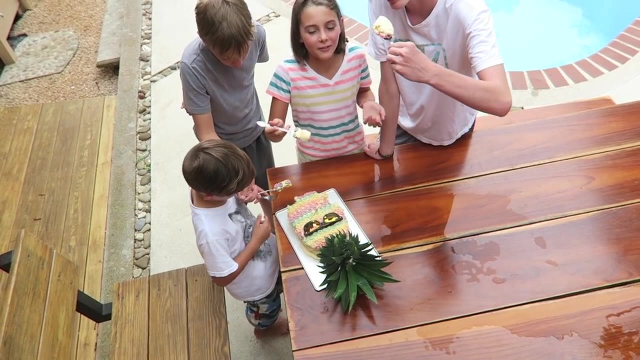 Thanks so much for joining me today, And don't forget to like, subscribe and comment down below if you like pool parties or pineapples more. Okay, okay, Oh, that was a lot of frosting. Oh boy, All I got was frosting. 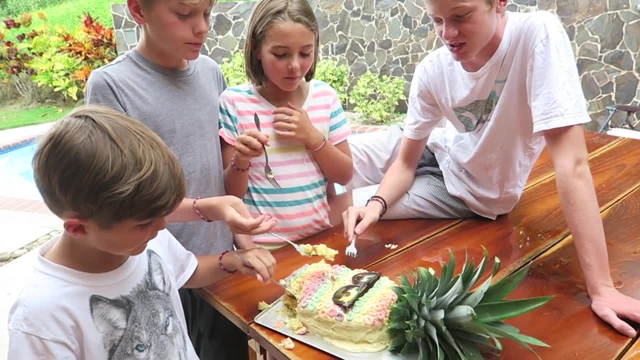 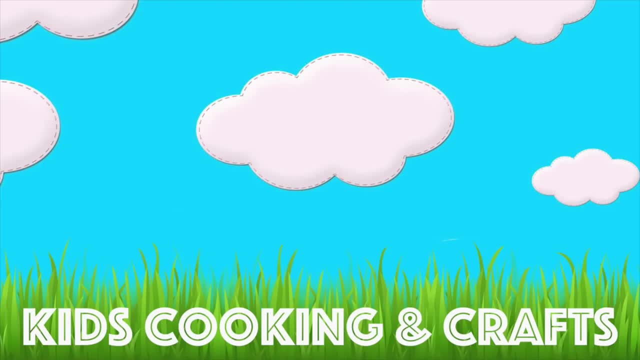 It tastes exactly like pineapple. Yeah, The frosting does That is really good. Thanks, Uh-huh, Mm-hmm. See you next time. Bye, Bye, Bye, Bye, bye.